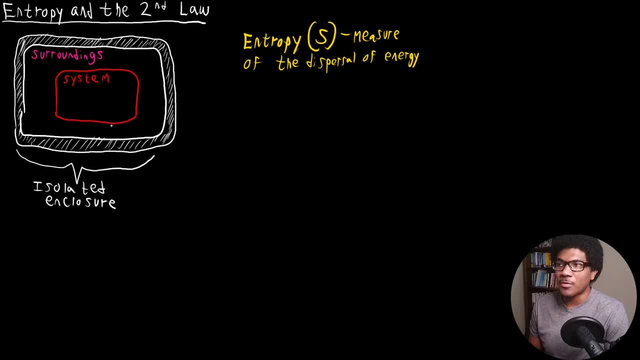 our surroundings and system enclosure, our general, you know, system defined in an isolated enclosure. Let's say, for this isolated enclosure there's some transfer of heat from the surroundings to the system, right? so it's set up in such a way that there can only be heat transfer between the system and surroundings, right that? 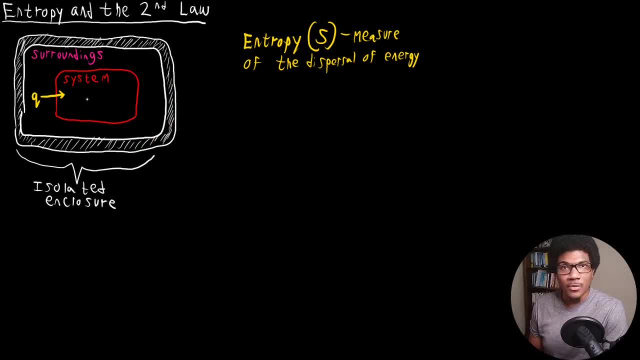 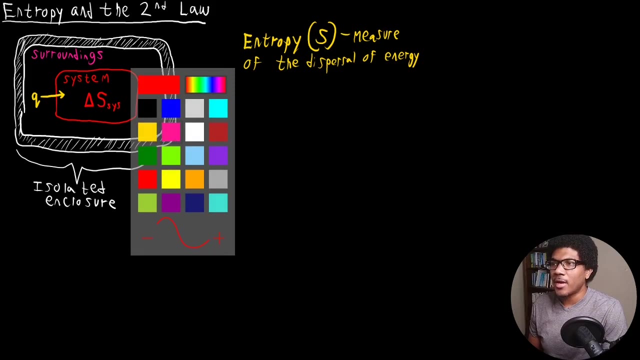 means that there's going to be some change in the dispersal of energy for the system, right, because it's receiving some energy from the surroundings, right? So you're going to have a delta S for the system and the same thing here for the surroundings, right? You're going to have some sort of change in its dispersal of energy, since. 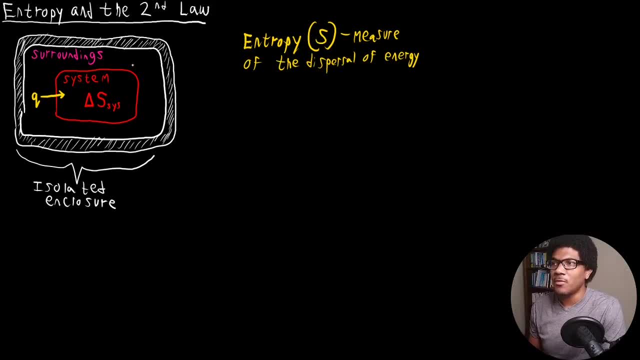 it's giving some of this energy to the system in the form of heat. right, So we're going to have a delta S for the surroundings as well. right, So you have a delta S for the system and a delta S for the surroundings. Now the second law of thermodynamics is related specifically to the 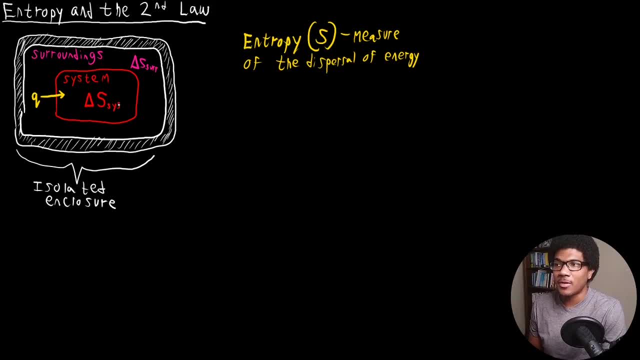 delta S of your entire universe, right. So you're going to have a change in delta S for the system, a change in delta S for the surrounding, and the sum of both of those gives you the delta S for your universe, right. So let's define delta S- universe. 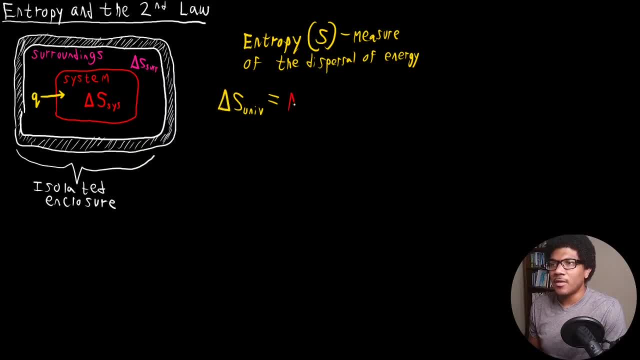 as being equal to the sum of delta S for your system plus the delta S of your surroundings. Now this is really crucial to understand That when we're talking about the second law of thermodynamics, we're really referencing the change in entropy for the universe, not just the system and not just the surroundings. 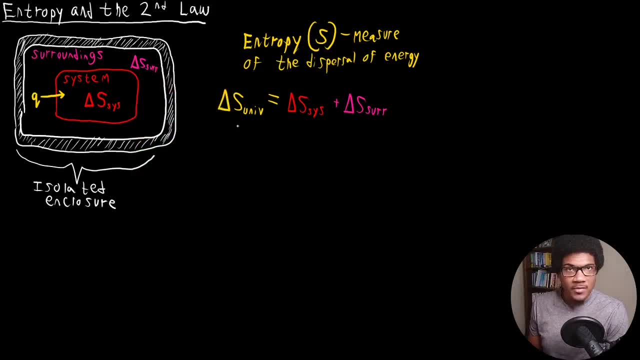 So what is the second law of thermodynamics? Well, the second law of thermodynamics tells us that there's always going to be a net increase in the delta S of the universe, right? So we'll have delta S. universe will always be greater than zero, right? So this? 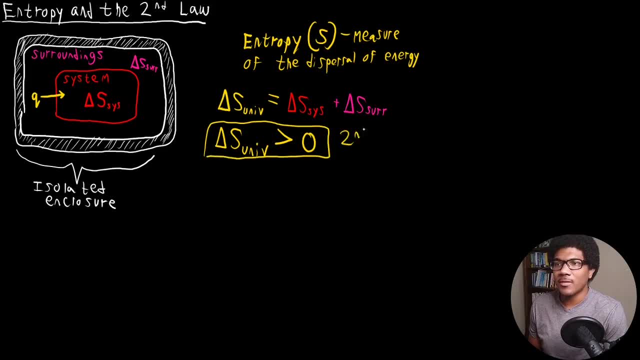 is the second law of thermodynamics right. So, like I said, basically this is just telling us that for any real process there will be a increase in the entropy right. So there's a few ways to state this right, So we can say that for any real process, 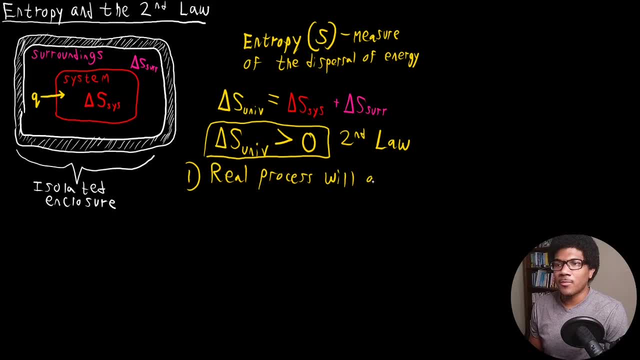 there will always be an increase in entropy. So, for instance, if we have a river in our universe, right- and this is why I'm saying that it's so important for you to understand that we're talking about delta s of the universe- You can have a decrease in entropy in the system or surroundings, respectively, right? 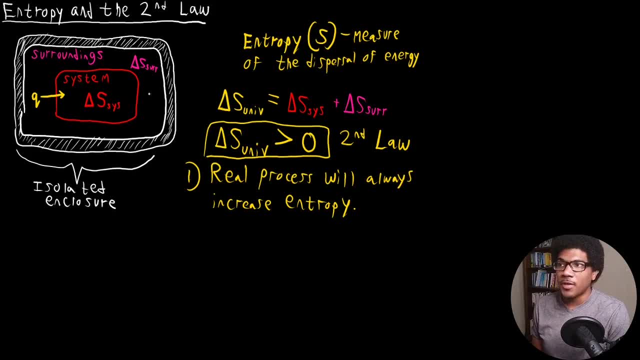 So, if we think about it here, right, with delta S surroundings, it's going to be donating some heat or transferring some heat to the system. And then the second law of thermodynamics is that we want to have a decrease in entropy, Right, So the entropy of the system is going to increase because that thermal energy is going to increase the fluctuations of the atoms. 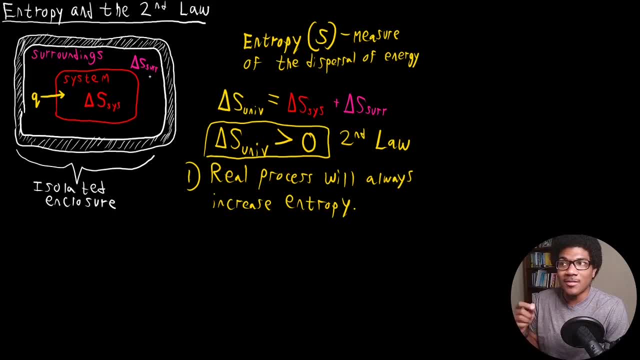 So it's going to increase the system entropy, but the surrounding entropy is going to decrease. What the second law of thermodynamics is saying is that there always will be a net increase, Right? So let me actually add that word here. It's always going to be a net increase in entropy, when you're talking about the entropy of the entire universe. 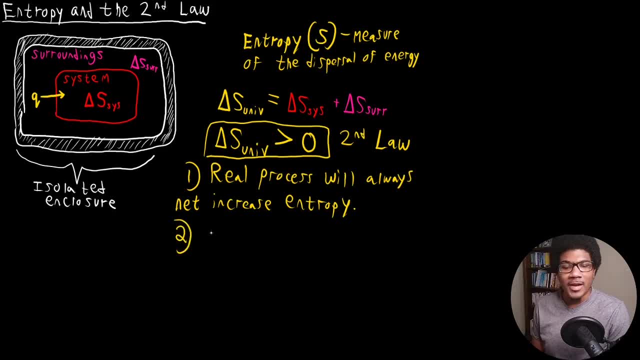 Now the other way to say. the second law of thermodynamics involves this idea of spontaneous change And basically this is just saying the same thing like a real process, Right? So for a spontaneous change, There will always be an increase in entropy. 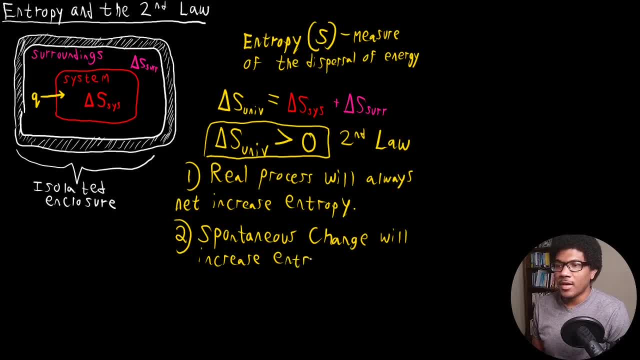 Will increase entropy In an isolated system, Right? So these are really two ways of saying the same thing, Right? So this first statement is just saying that any real process will have a net increase in entropy, But the other one kind of gets to what we talked about about spontaneous change. 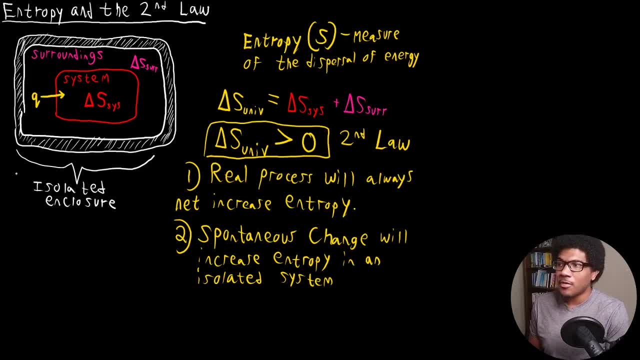 So now the question kind of remains here: How do we thermodynamically Define entropy, Right? So think about it, as we're trying to measure the dispersal of energy, Right, And we have a useful way of tracking how energy is dispersed or transferred by heat.